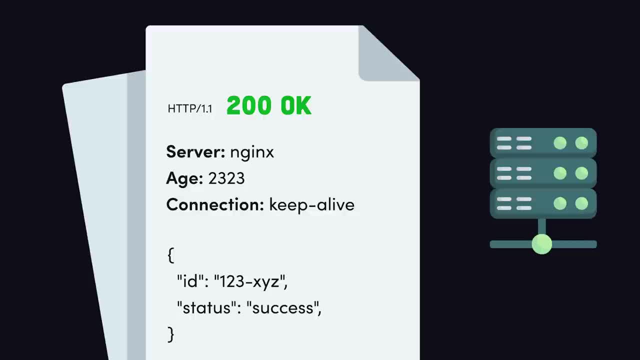 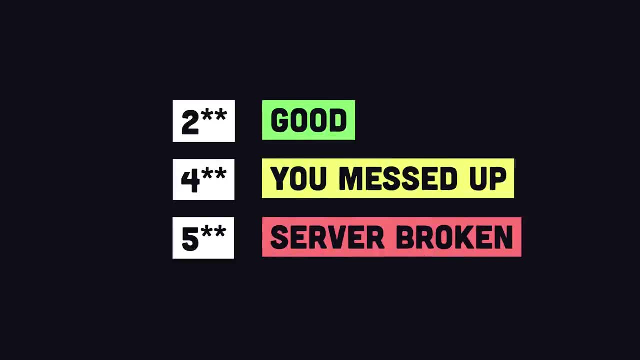 formatted into a response message. the top of the message contains a status code to tell the client what happened to their request. codes at the 200 level mean that things went well, at the 400 level it means something was wrong with your request and at the 500 level it means 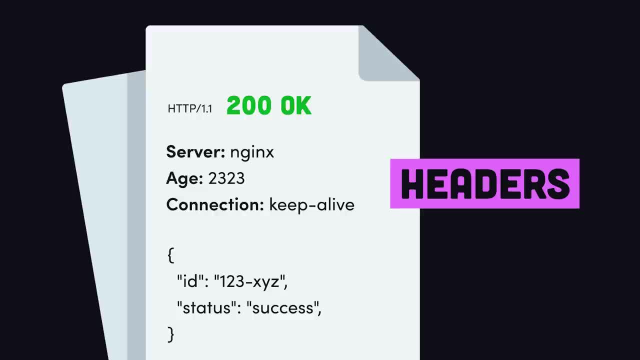 that the server failed. after the status code, we then have the response headers, which contain information about the server. that's followed by the response body, which contains the data payload and is usually formatted in JSON when talking about api's. now, an important part of this architecture is that it's 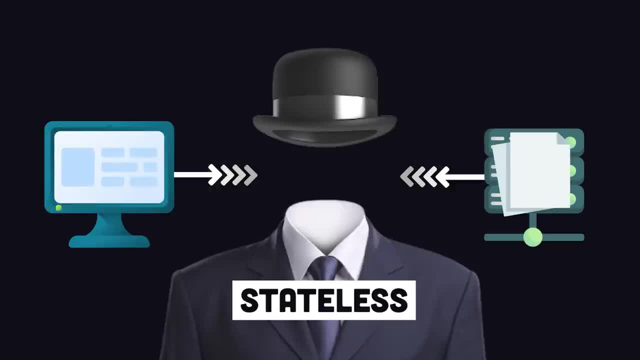 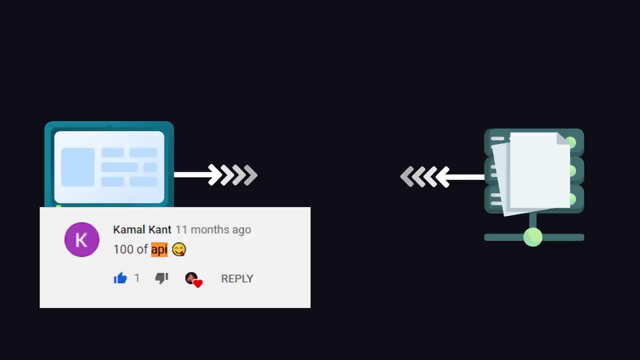 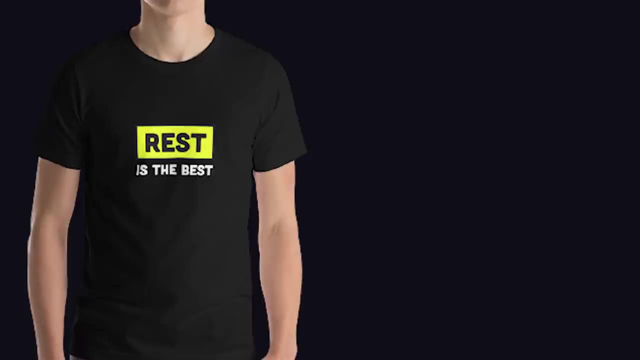 stateless, which means that the two parties don't need to store any information about each other and every request response cycle is independent from all other communication, and this leads to well-behaved web applications that are predictable and reliable. this has been interesting to me and I hope you enjoyed this video and I'll see you in the next. 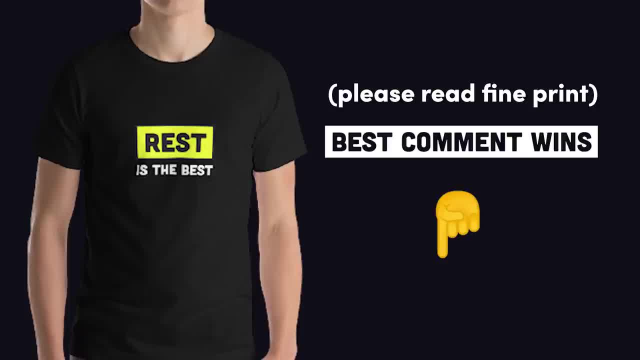 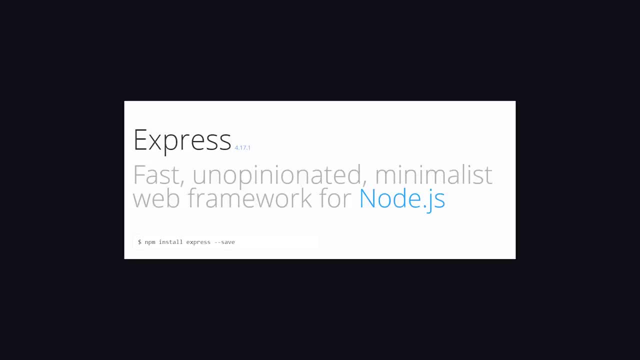 video. next week I'll pick out the best one to win this free t-shirt. and now it's time to go beyond 100 seconds, to build a restful API from scratch. the most popular framework for building restful API's and node is ExpressJS. it's been. 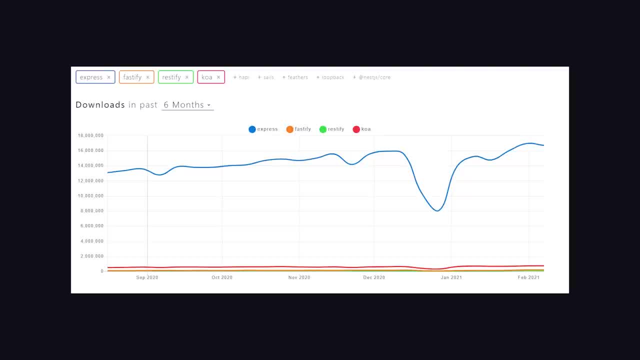 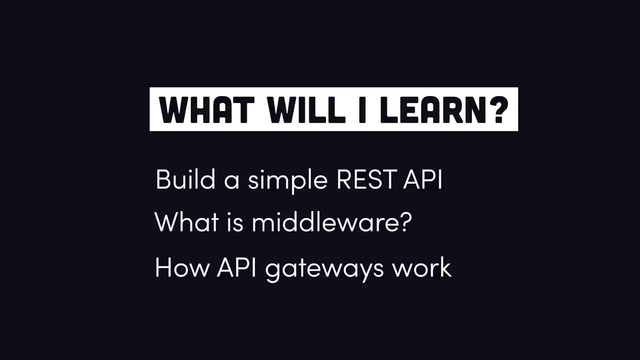 around forever, and it's very minimal and easy to learn if you know a little bit of JavaScript. over the next few minutes, we'll use Express to build our own restful API from scratch. you'll learn how to create different endpoints for your API. we'll also show you how to use it in a future video, so until then, stay. 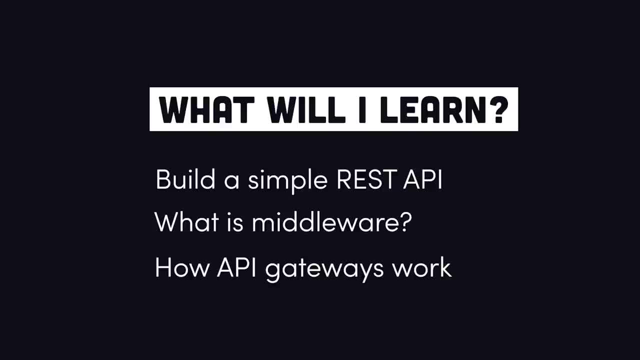 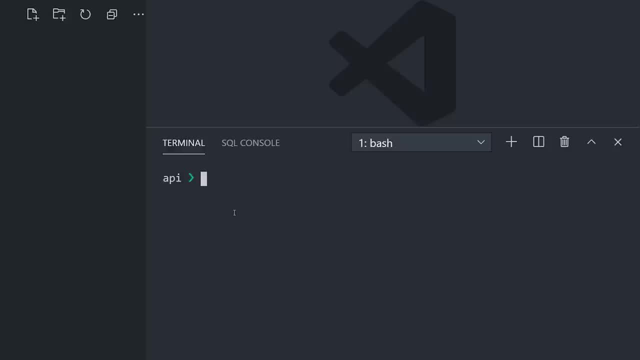 tuned. also look at slightly more advanced concepts like middleware and tools in the cloud for deploying your API, like API gateways. to get started, you'll want to open up VS code to an empty directory. you'll need to have nodejs installed and I'm using version 12 for this video to start a new node project. let's run. 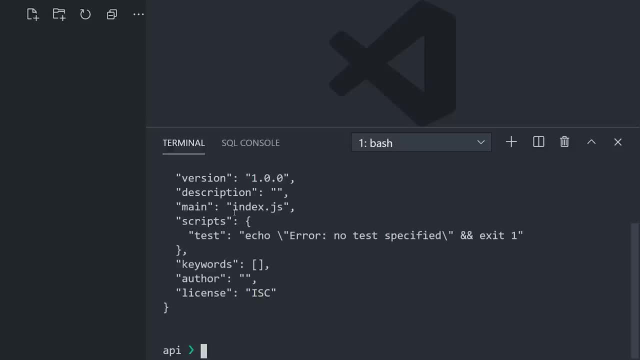 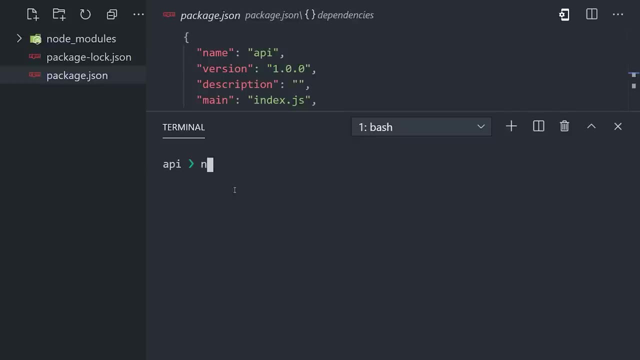 npm init y from the command line. this will create a package JSON and give us a context for installing packages that we can use in node like Express. let's go ahead and install Express using npm installjson. I'm going to go ahead and install Express using npm installjson. 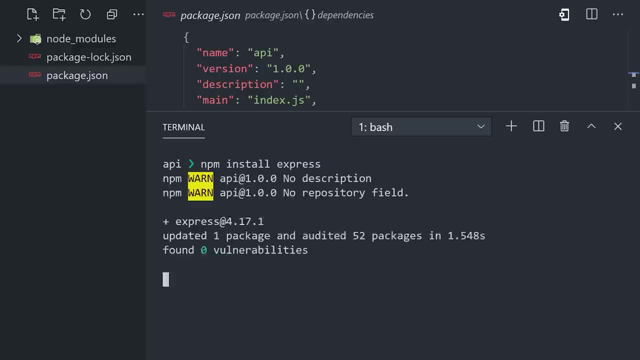 I'm going to go ahead and install Express using npm installjson. I'm going to go ahead and install Express using npm installjson. you'll notice that adds Express to our dependencies in the package JSON file. from there we'll need a file to write our code in, so let's create an indexjs. 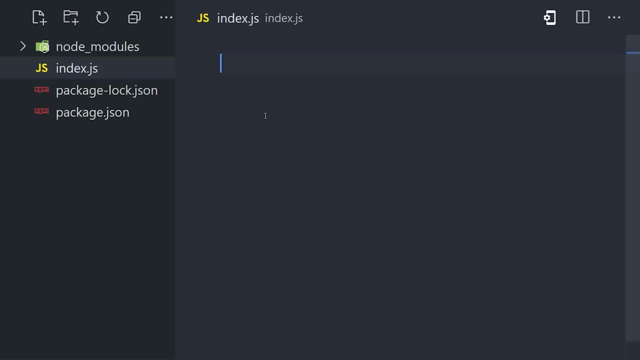 file. at the top of that file we'll declare a variable for app, which represents the actual API that we're building, and its value is an import of the Express package, which itself is a function, so we'll add parentheses after it to initialize it now. at this point, our API hasn't defined any endpoints, but 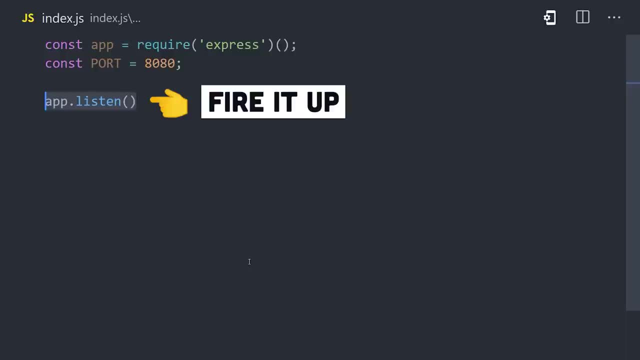 let's go ahead and run it anyway. the way you find the API is by going to the API server, and the way you fire up your API on the server is by calling app dot listen. that tells it to listen on a specific port which we've defined as its own separate. 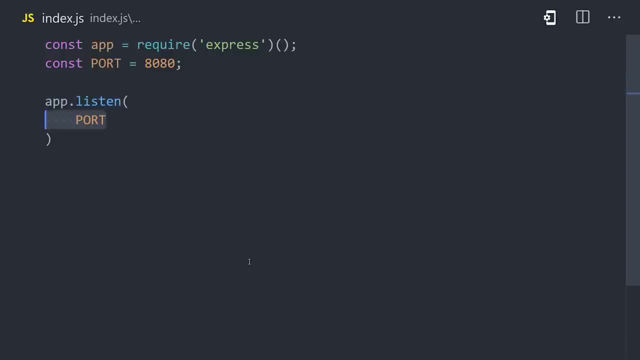 variable as 8080. then as an optional second argument to listen, we can fire a callback to let us know when the API is ready and we'll just have it. console log: the main URL. we can now run the API by going to the terminal and running node period to run that indexjs file. 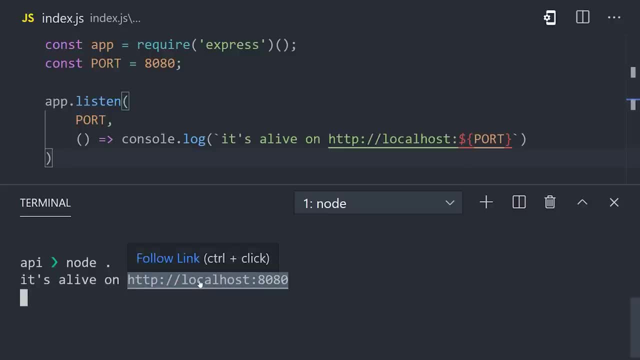 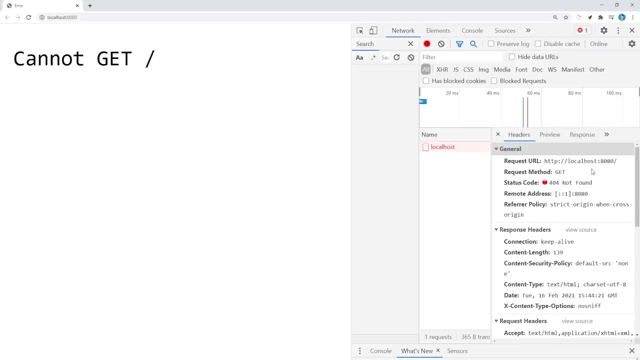 and it should console log. it's alive on localhost 8080. if we paste the URL into the browser browser, you can see we get a message of cannot get. That's because we don't have any API endpoints set up yet, but Express is still responding with an error message. In fact, you can open up the. 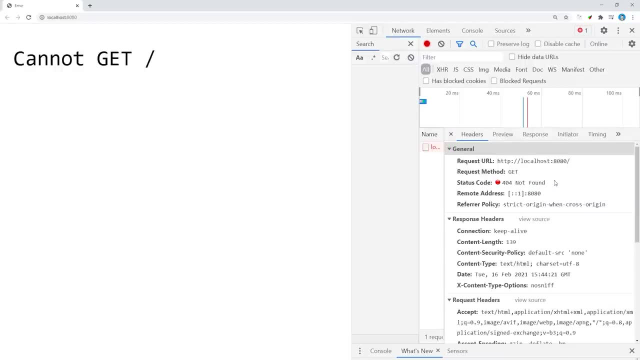 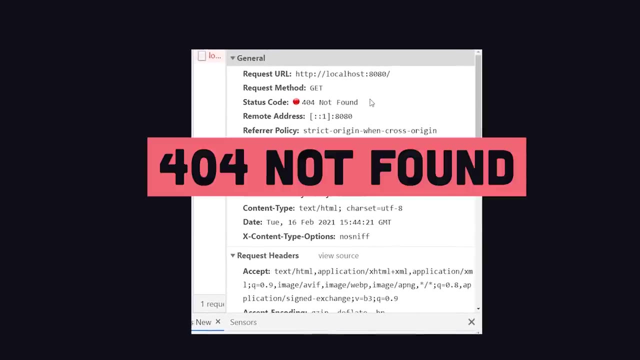 network tab in Chrome. If we look closely, we can see that our server responded with a 404 status code, meaning that page was not found. At this point we know our API is working, but debugging it in the browser is usually not the best option. There are many different ways we can access our 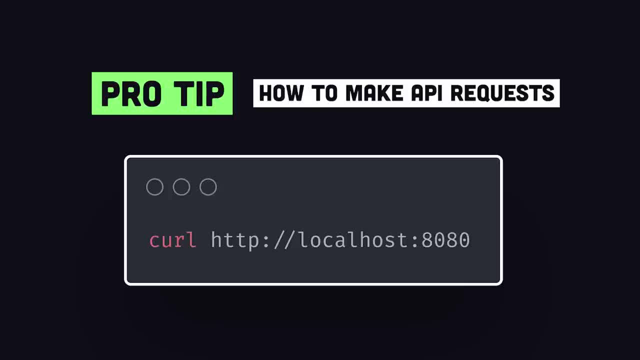 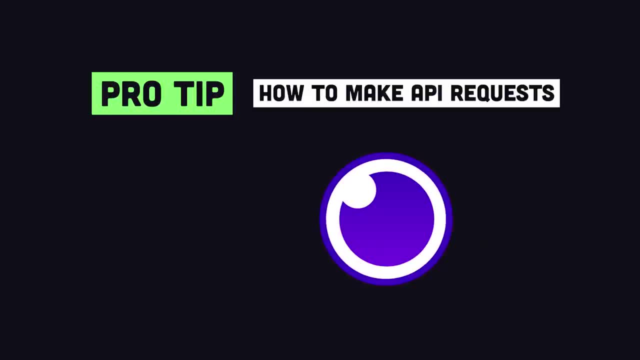 API. We could use curl from the command line, we could install a VS Code extension or we could use a REST client like Insomnia or Postman. I'm going to be using Insomnia throughout the rest of this video because it provides a really nice way to format your requests and also view a history. 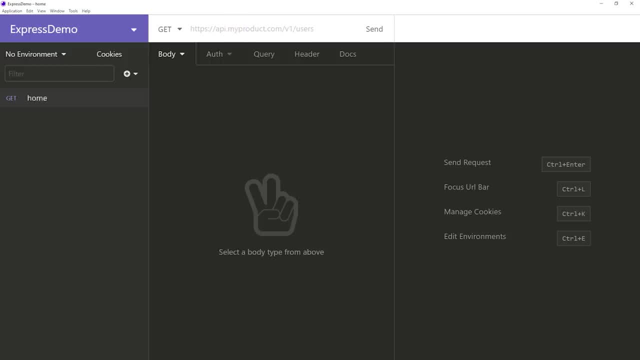 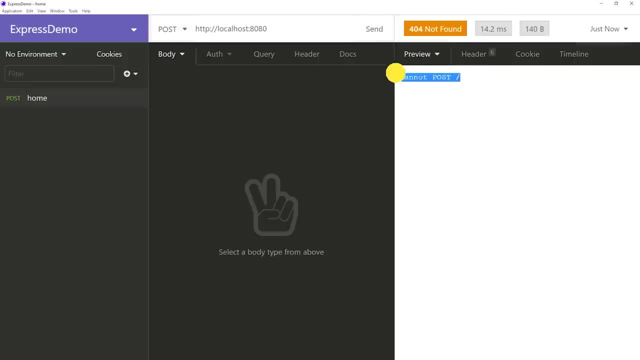 of all your interactions From Insomnia. we can create a new request, then simply paste in our URL. We can easily change the HTTP verb from the drop-down menu here, click send and then get the response in a nicely formatted, developer-friendly way. We can even see the timeline. 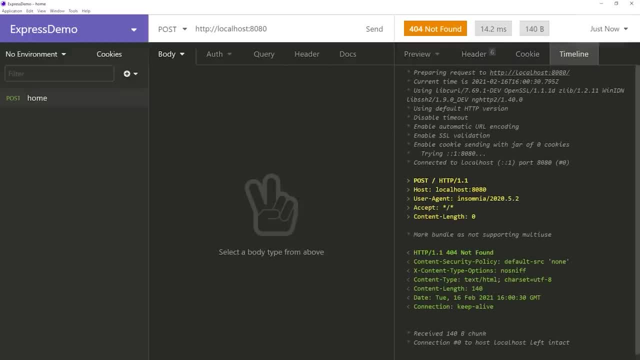 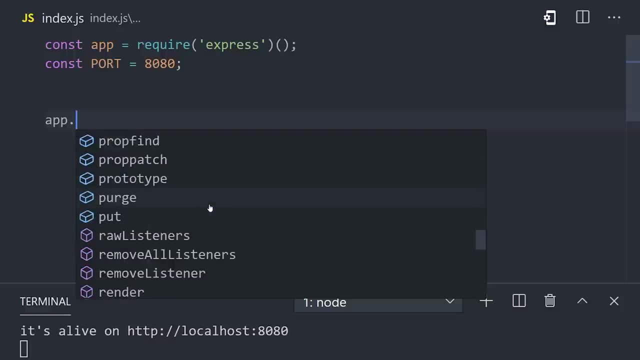 here with our request in yellow and the response in green. But now we need to get back to our JavaScript and add an endpoint to the API. We can do that by chaining an HTTP verb to the app instance. If you type a period after app, you'll get IntelliSense on a bunch of different methods. 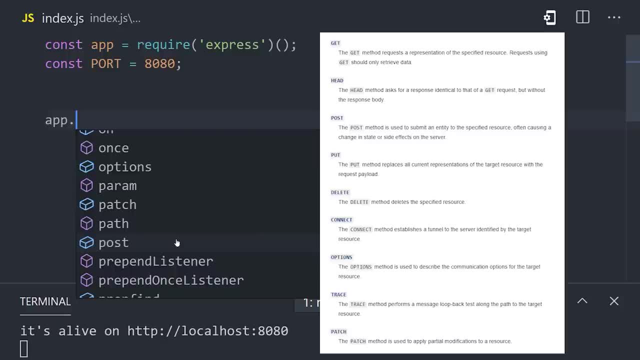 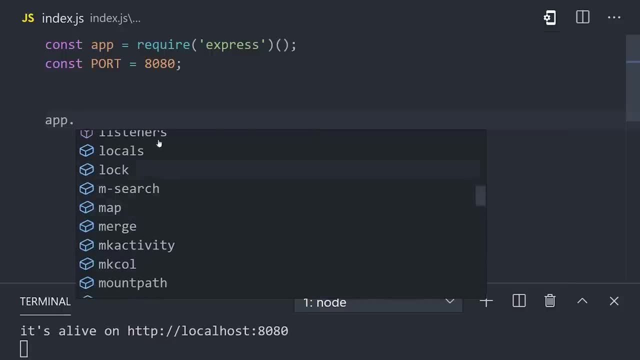 that live on this object and you'll notice methods for get, post patch, etc. which represent different HTTP verbs. If we want to add a get endpoint to the t-shirt URI, we can do that by passing slash t-shirt as its first object. 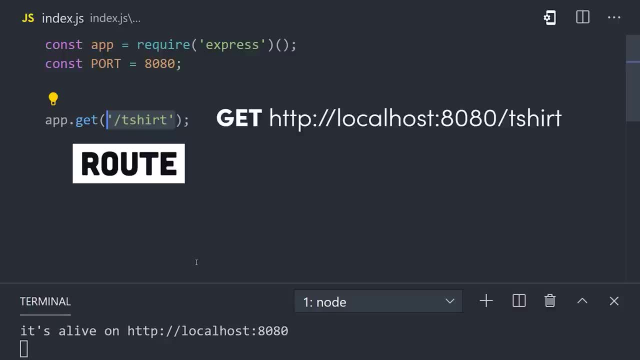 That'll automatically set up our server with that endpoint. Then it's our job to handle a request to it, which we do by passing a callback function as the second argument. Whenever a client or end user requests that URL, it will fire this callback function to handle the request, The function. 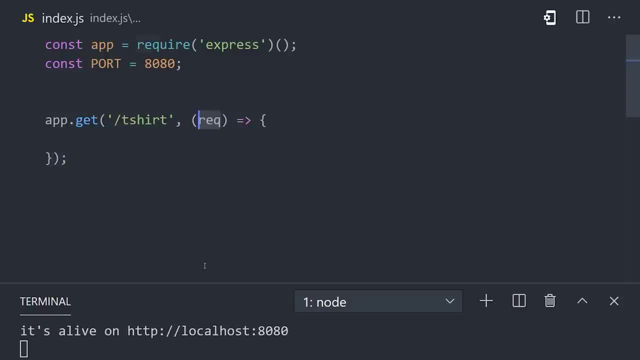 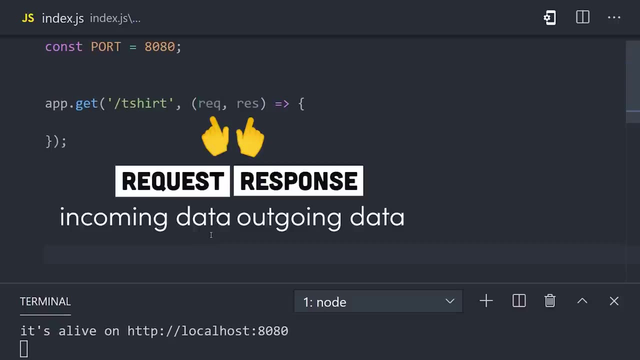 itself provides access to two different objects: the request object and the response object. The request is the incoming data, while the response is the data we want to send back to the client. The most important thing it does is allow us to send a response back to the client. That response can have a status code. 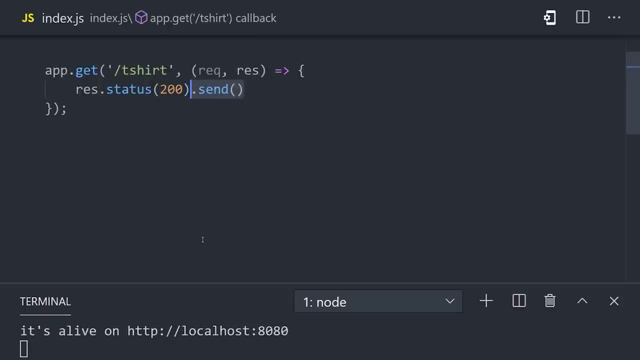 like 200, for an OK response, Then we can send a data payload along with it. If we pass a JavaScript object as the argument, then it will send that data back as JSON by default. Let's go ahead and save the file, then restart the server from the terminal. 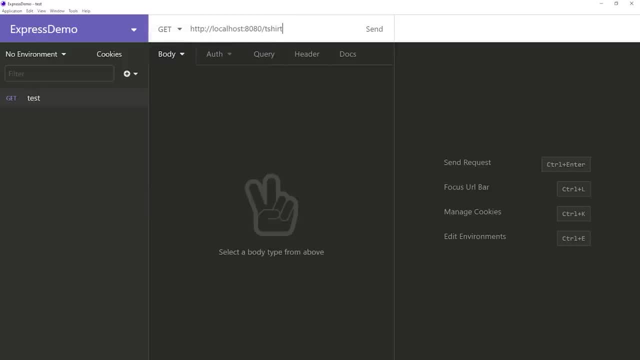 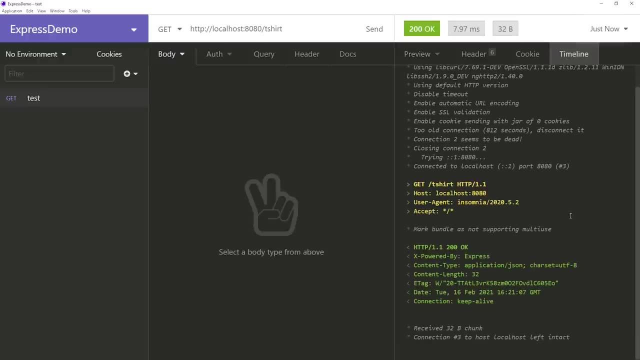 From Insomnia. we can then make a get request to localhost 8080 slash t-shirt. When we do that, we get a JSON object back as the response body With a status code of 200.. That's pretty cool, But now let's go back to our code and add a second endpoint. 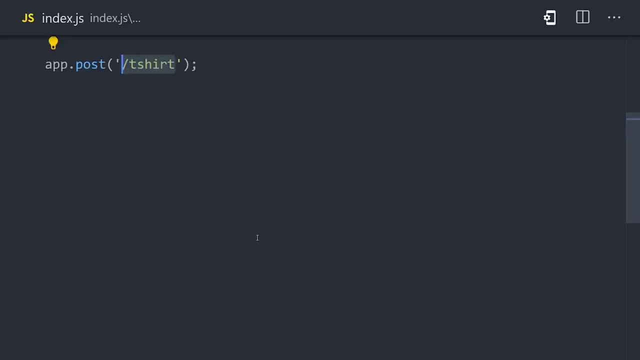 this time a post endpoint followed by a slash and a dynamic URL parameter that represents the ID of that t-shirt. There might be millions of different t-shirts on this API and a dynamic URL allows us to handle all of them from a single function When dealing with a post request it. 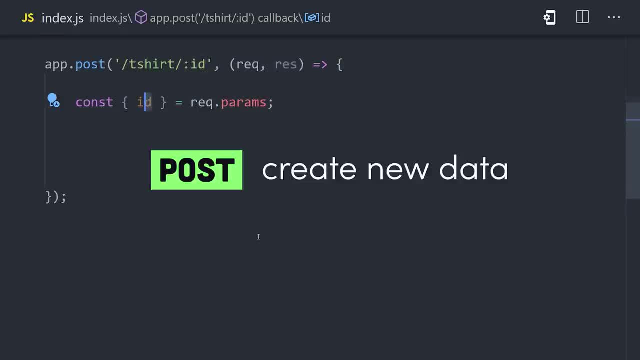 means that the user is trying to create new data on the server, or create a new t-shirt. in this case. First, we need the ID, Which we can get from the URL, and its value is made available to us on the request parameters object. Second, we also need a logo for the t-shirt. 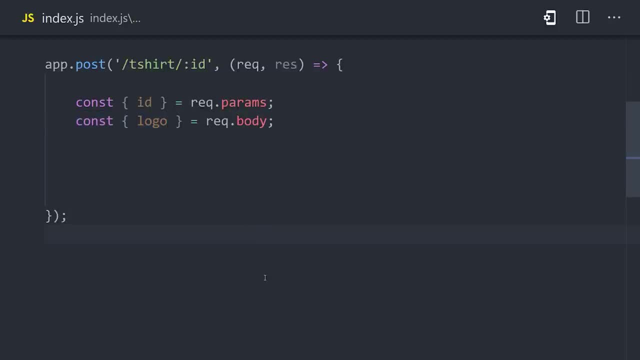 But the logo is contained in the request body which, if you remember from earlier, is a custom data payload contained in the incoming request. In other words, the request object in express allows us to access information from the request message, like the URL, parameters, the body, the headers, etc. And now that we have that information, 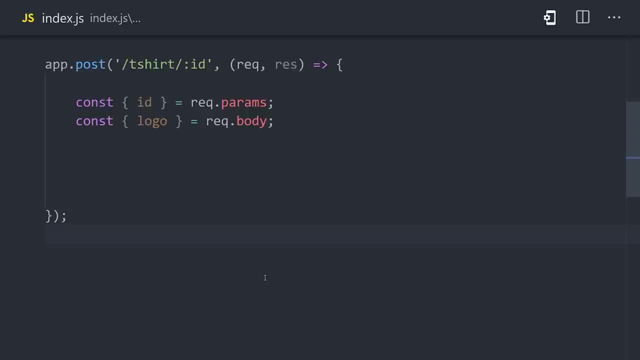 we could use it to name our data, and we could also use it to name our data in the form of a save, a new record to the database, or something along those lines. That's beyond the scope of this video. What we'll do for right now is check to make sure that we have a logo in the request. 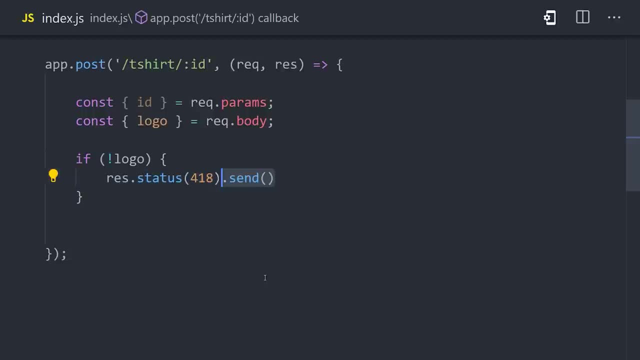 body, and if we don't, then we'll send an error response with a 418 status code and an error message that we need a logo. But assuming we do have a valid logo, we can just send a response with a t-shirt that contains that logo and ID. Now let's go back to Insomnia and we'll make a 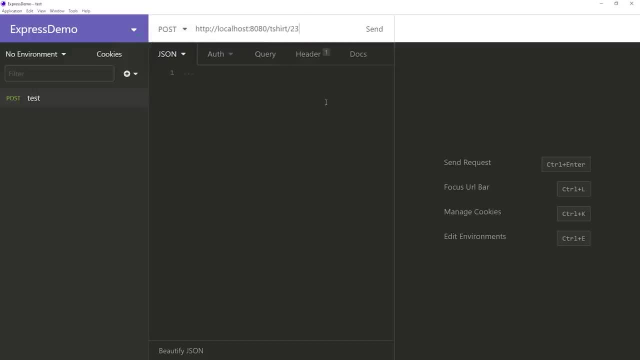 request to the t-shirt endpoint, followed by a unique ID. That can be whatever you want. Then in the body section we'll go ahead and add a request body with a format of JSON and it's just a JSON object that contains a logo with a string value. If we send that request, you'll notice we. 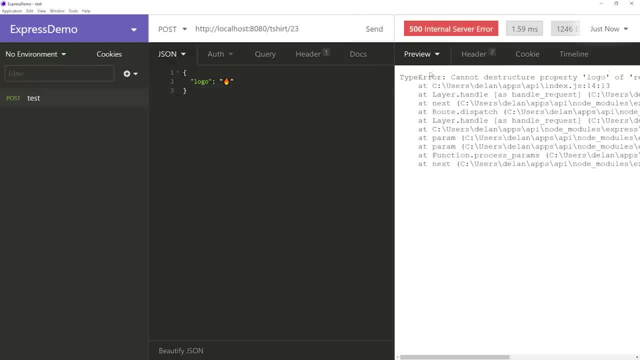 get a 500 error response, which means our API code is broken. So what's going on here? It's telling us we have a runtime error because we can't destructure the property logo from the request body. The reason for that is that Express 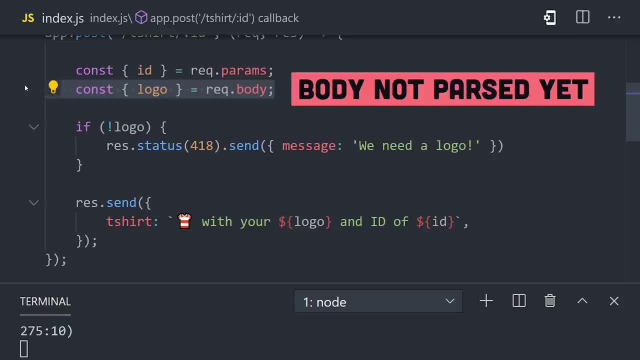 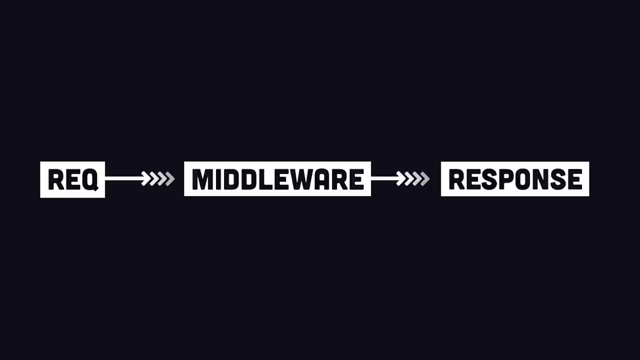 does not parse JSON in the body by default. Not everybody uses Express to build a JSON API, so that's not the default behavior. What we need to do here is set up middleware that tells Express to parse JSON before the actual data hits. the function that we're using here to handle the 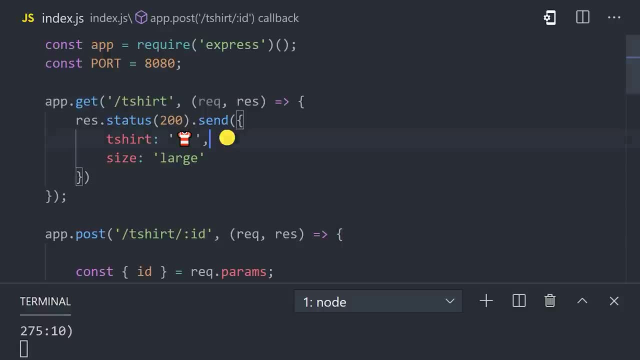 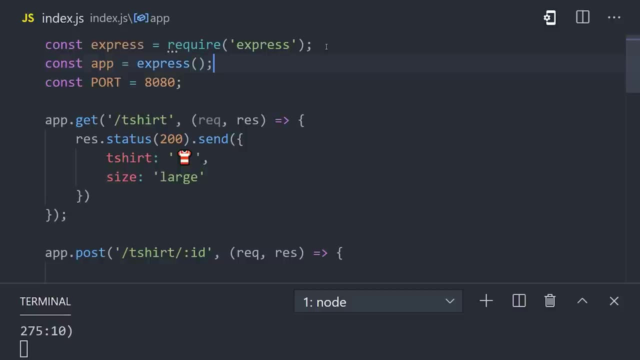 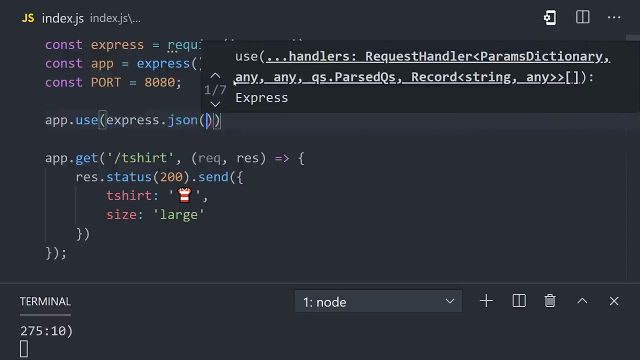 request. When you hear the term middleware, think of shared code that runs before every endpoint callback that you've defined. Very common middleware is built into Express itself. We can refactor our code here a little bit to make a variable for Express And then we can call appuse to apply middleware, In this case the middleware we want to apply. 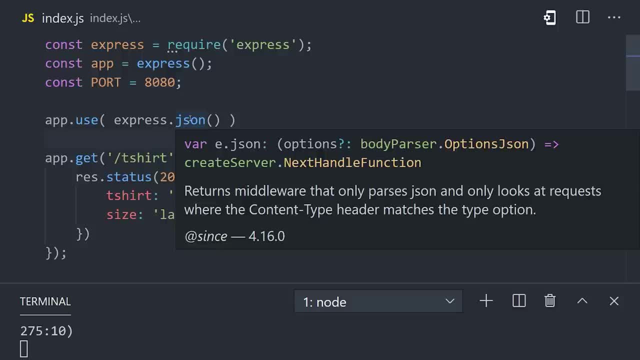 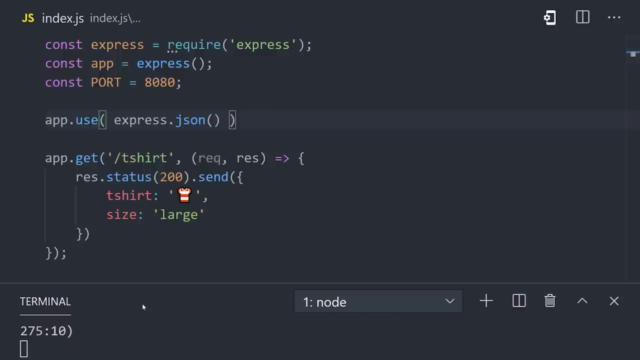 is the expressjson middleware. Now, every request that comes in will first go through this express JSON middleware, which will convert the body to JSON, therefore making it available in our post callback. Let's go ahead and save, restart our server and then go back to Insomnia. And if we 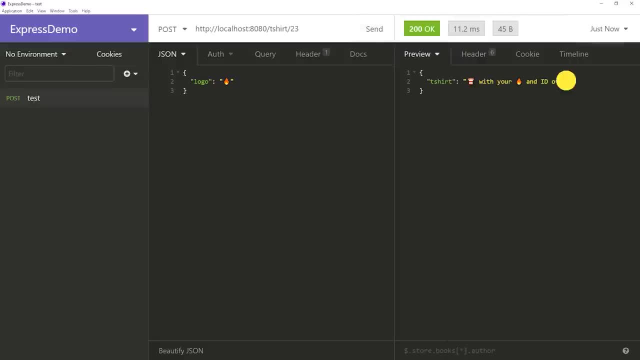 send the same exact request. you'll notice this time we get back a successful response. In addition, if we make the logo an empty string and try to send the same request, we get a 418 response, along with a message that we need a logo. Congratulations, you just built a RESTful API from scratch with Nodejs and Express.